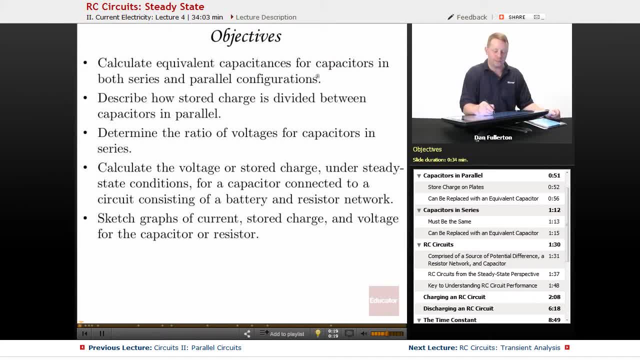 So our objectives include calculating equivalent capacitance for capacitors in series and parallel configurations. we've done that before. we're just going to review it a little bit: describe how stored charge is divided between capacitors in parallel. determine the ratio of voltages for capacitors in series. calculate the voltage or stored charge under steady state conditions for a capacitor connected to a circuit consisting of a battery and resistor network. and finally, sketch graphs of current stored charge and voltage for the capacitors in series. 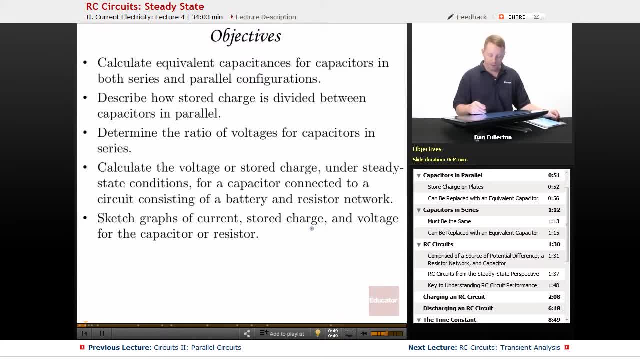 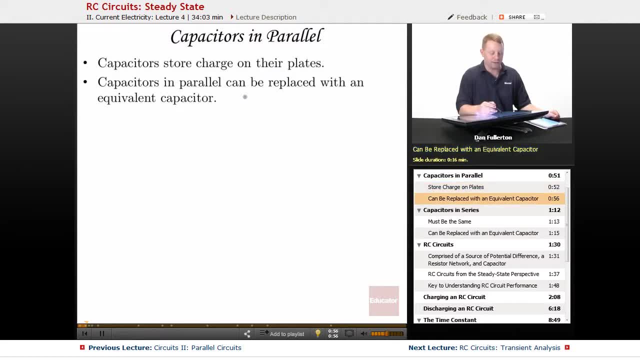 So very quickly, let's review capacitors in parallel. We know capacitors store charge on their plates and capacitors in parallel can be replaced with an equivalent capacitor, And we talked about doing that. the equivalent capacitance for capacitors in parallel is just the sum of the individual capacitances. 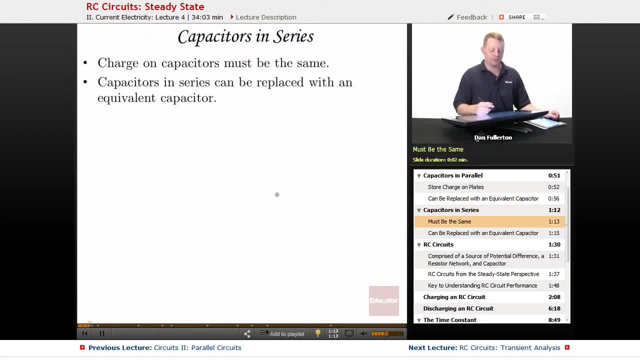 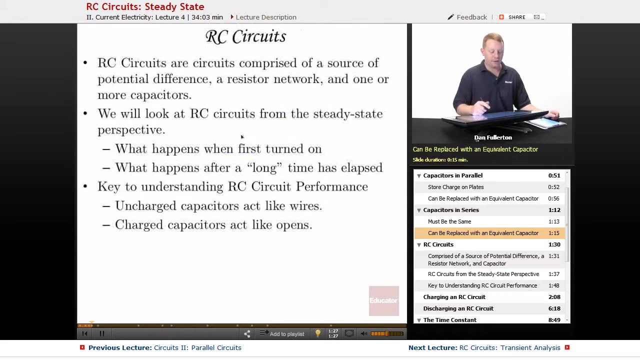 And for capacitors in series. the charge on them must be the same and they can be replaced with an equivalent capacitor. So as we get into RC circuits specifically, then RC circuits are comprised of a source of potential difference to make the current flow, a resistor network and one or more capacitors. 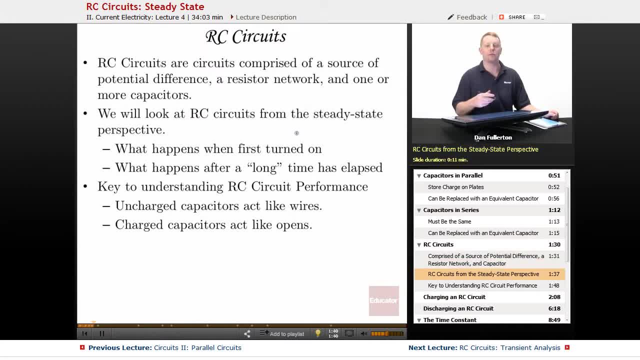 We're going to look at RC circuits from the perspective now of what happens when they're first turned on and what happens after a long time and what's in the middle. we're going to leave until the next lesson, at least for now. starting out Now, the key to understanding RC circuit performance. Uncharged capacitors. 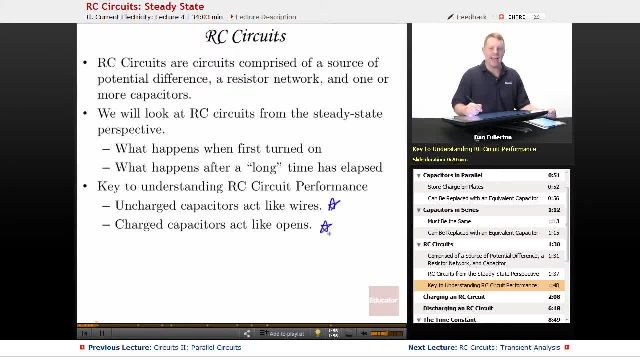 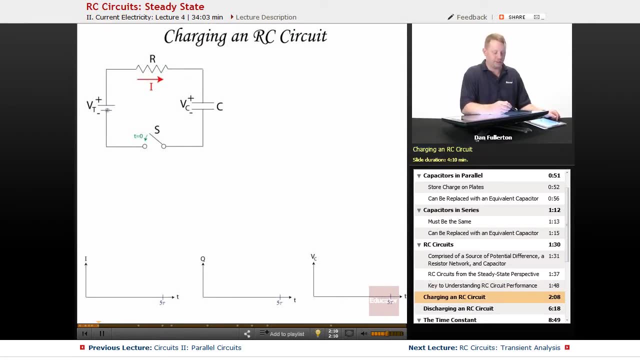 act like wires. Charged capacitors act like opens. Gotta know these two facts. It's going to help you immensely with your analysis of capacitor circuits. So let's take a look at charging an RC circuit. Here we have a source of potential difference. 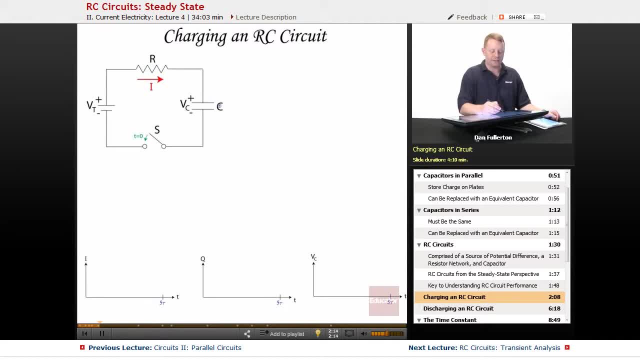 some VT. We've got a resistor R, We have a capacitor C and we've defined the positive and negative side of our capacitor And at time T equals zero. we're going to close this switch and see what happens Now. initially, the capacitor acts like a wire when it's uncharged. 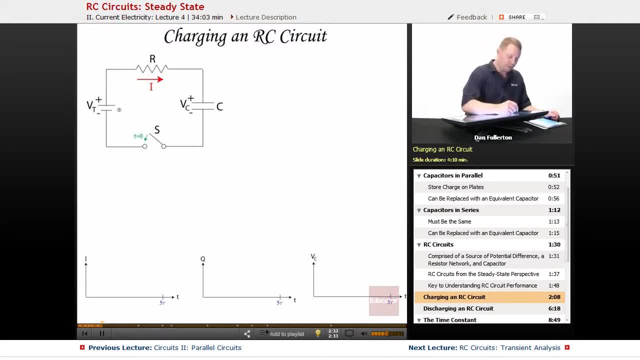 So if we were to take a look at this and we're going to follow a Kirchhoff's voltage law path around, that way, I could write that minus VT- because starting here we see the negative side first, plus IR, plus the voltage across our capacitor is going to equal zero All. 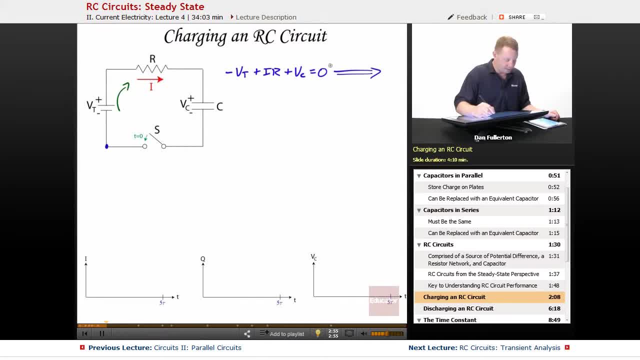 right? Well, we also know that our capacitor is charged divided by voltage, voltage across our capacitor. Therefore, the voltage across our capacitor is Q divided by C. So I can rewrite my equation as: minus VT, VT plus IR, plus Q over C must equal zero. But we also said at time: T equals zero when. 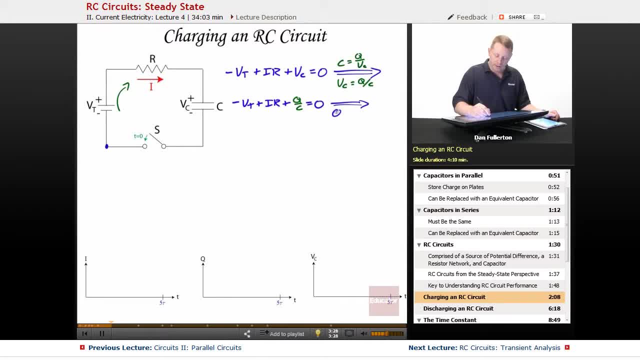 we first close that switch, the charge on our capacitor is going to be equal to zero. It's uncharged. So that simplifies our analysis a little bit. And we have: minus VT plus IR equals zero, Which implies that VT equals IR- Probably not a surprise VC- therefore must equal zero. 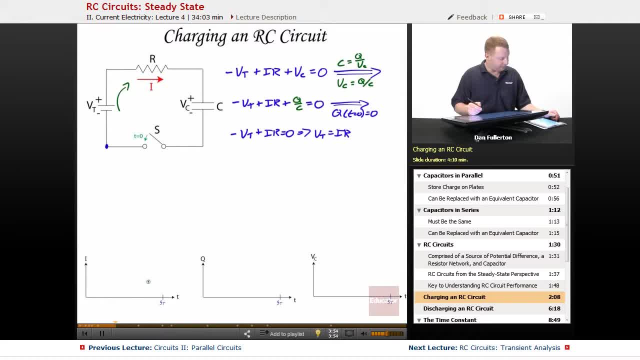 So if we were to do our plot of the different things we have down here, initially the current flowing through our circuit is going to be VT over R, So we can make one point over here for the current through our circuit and call that VT over R. at time equals zero. We also 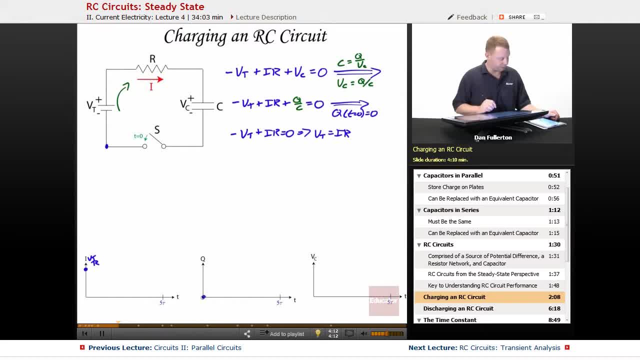 know the charge on our capacitor at time equals zero. So we can make one point over here for the current through our circuit and call that VT over R. at time equals zero. And we also know the voltage across our capacitor. because Q is zero must start at zero. 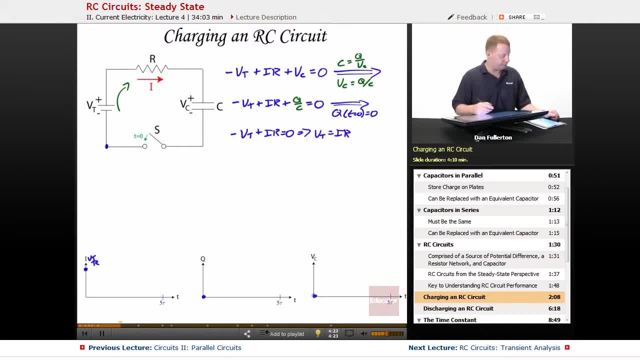 So there's our initial analysis. Now let's take a look and assume that the thing's charged up. It's been a long, long, long time, And a long, long, long time is something we're going to define here in a couple minutes. 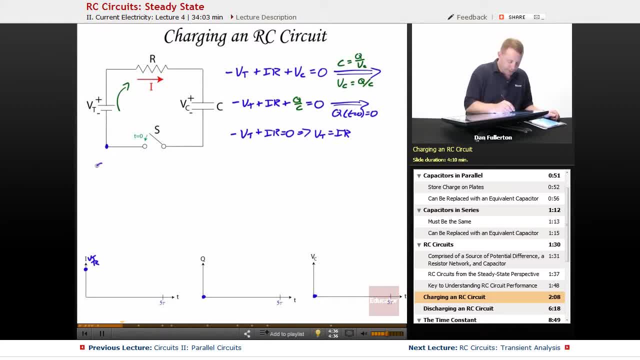 But now, after a long time, the switch has been closed for a while. the capacitor now acts like an open. It doesn't allow current Current to flow. So as T approaches infinity, as it gets very big, and we apply Kirchhoff's voltage law,